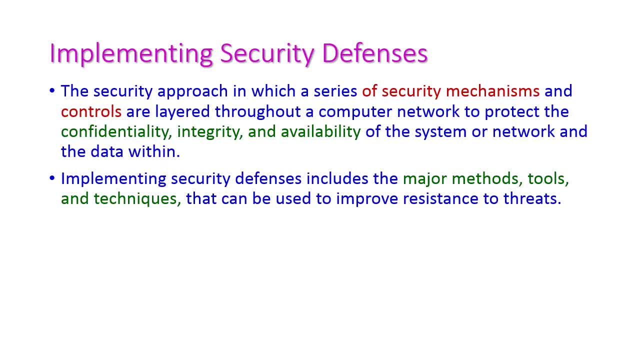 So implementing security defense. that means the security approach in which a series of security mechanisms and controls are layered throughout the computer network or throughout the computer system to protect the confidentiality, integrity and availability of the system resources or networks and the data or information which are stored in the system or network. 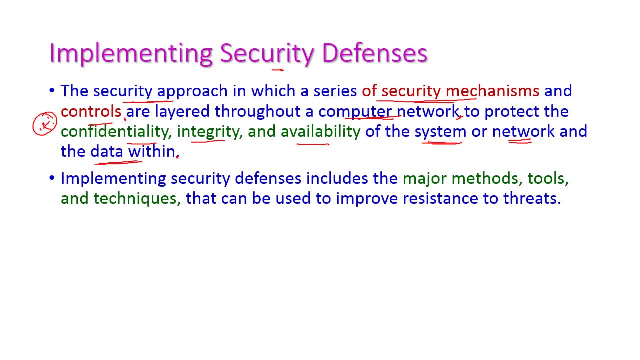 So let us see all those things one by one. So we have to protect all our resources from the threats. For that we need to implement the security defenses, And the implementing security defense includes the major methods, tools and techniques that can be used to improve resistance to threats. 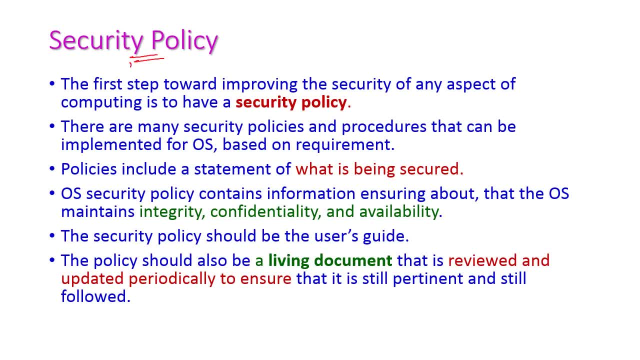 Security policy. This is the first step of improving the security of any aspect of computing. So the security policy is very important and there are many different types of security policies and procedures. based on the operating system and based on the requirement, the policies may be different. 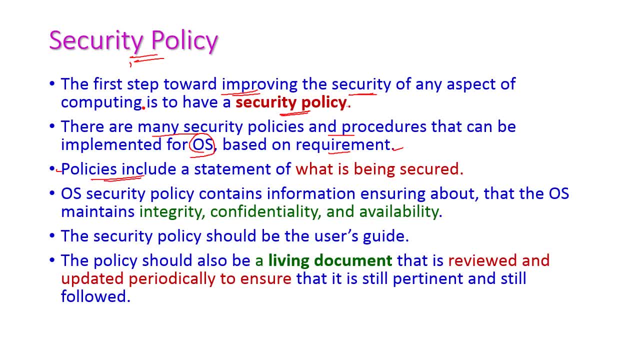 And the policies include a statement of what is being secured, What is secured and how it will be secured. Everything will be explained in security policy, because the security policy is simply a document. Okay, And why? a security policy which contains the information ensuring about that the operating system maintains integrity, confidentiality and availability? 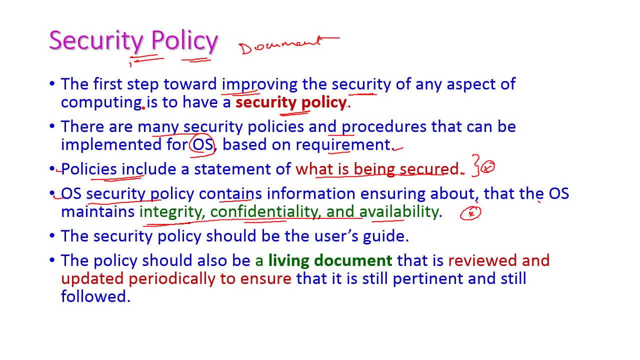 Okay. So if we give security for these things, then we can trust the particular operating system. Okay, That is. integrity, confidentiality and availability should be maintained in every operating system. Okay, And the security policy should be the user's guide. Okay, And the policy should also be a living document. that means it reviewed and updated periodically to ensure that it is still pretended and still followed. 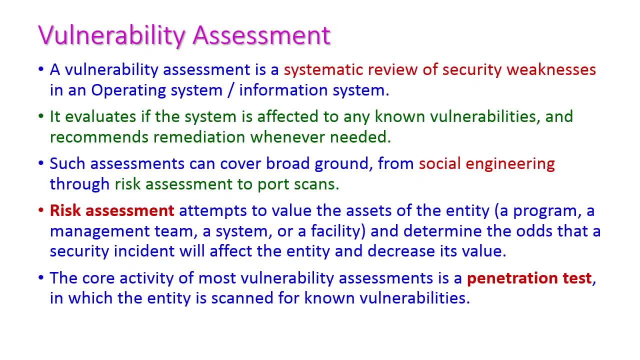 Okay. Vulnerability assessment: Okay, It is a systematic review of security weakness- Okay, In an operation, operating system or information system, that is, vulnerability assessment means a systematic review of security weakness. okay, and it evaluates if the system is subjected to any known vulnerabilities. 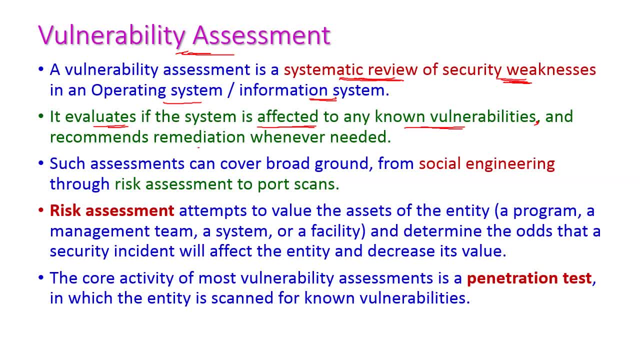 and it recommends the remediation whenever required. okay, and this is the duty of vulnerability assessment and this assessment can cover broad ground, from social engineering through risk assessment to port scans, right and risk assessment that will value the asset of entity. the assets here are the programs, management teams, systems and facility. these are assets and 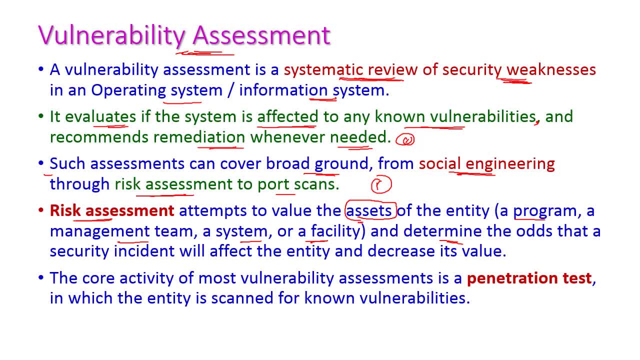 determine the odds that a security incident will affect the entity and decrease its value. that is, if the assets are affected, then what is the risk assessment? to port scans right and risk assessment that will value the asset of entity, decreased value of this asset and that should also be calculated and that will come under risk. 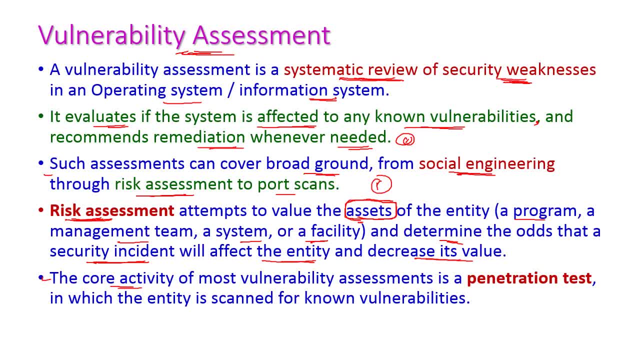 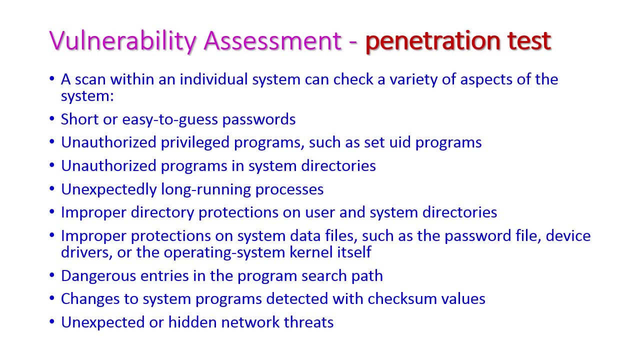 assessment. okay, the core activity of vulnerability assessment is penetration test. okay, this is very important, and in which the entity is scanned for known vulnerabilities. in the penetration test, a scan within individual system can check the variety of aspects of the system. okay, the penetration test will scan the system. uh, the following aspects, whether short or easy to guess. 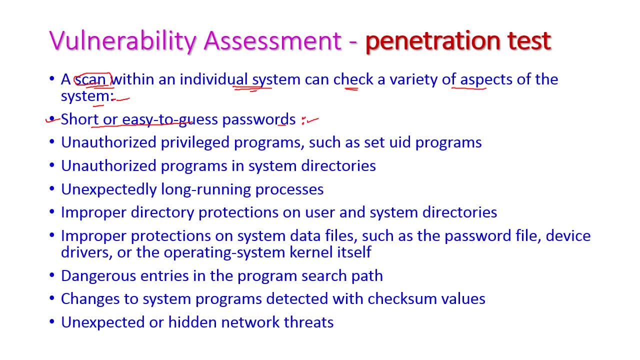 passwords if the passwords are easy to guess in the system. are unauthorized privileged programs such as setting user id programs- if there is any automatic setting of user id programs instead in our system or not, and unauthorized programs in system directories- unexpectedly wrong running process and improper directory protections on user and system directories- improper protections. 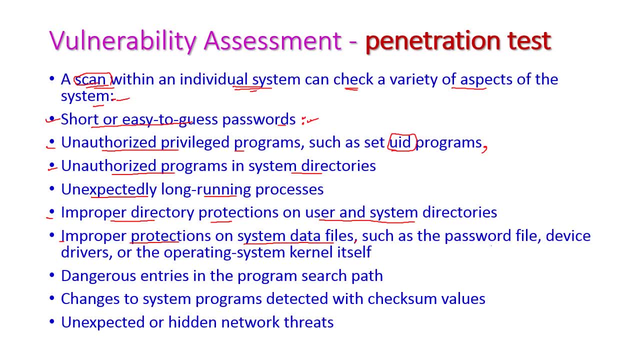 on the system, data files such as password files, device drivers or operating system kernel itself, and dangerous entries in program search path, change to system programs and so on. so these are the things we need to scan in this vulnerability assessment. so these are the things we need to scan in this vulnerability assessment. 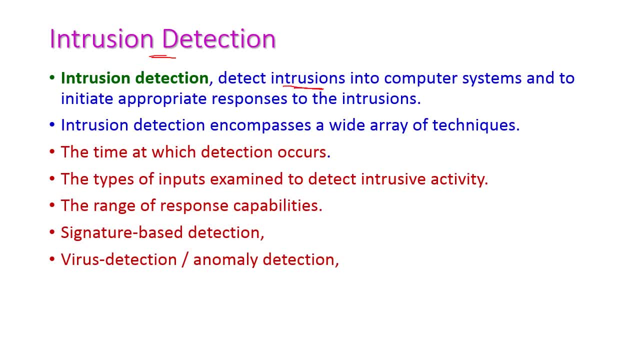 intrusion reduction. it detects intrusions into the computer system or into the network and to initiate appropriate response to that intrusions. this is intrusion deduction and there are varieties of techniques there in this intrusion deduction. first one, the time at which the deduction occurs and second one, the type of 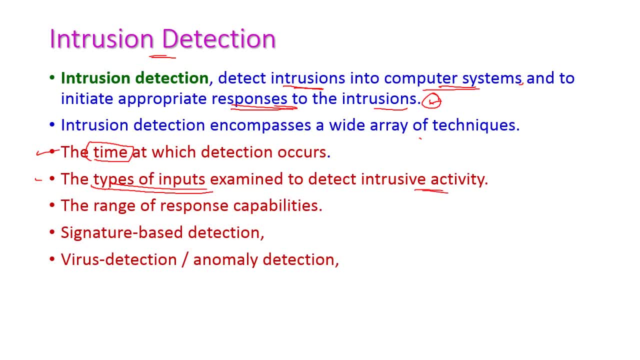 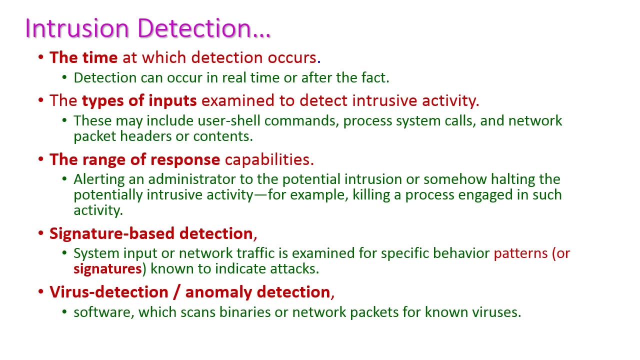 inputs examined to deduct the intrusive activity and the range of response capabilities: signature based deduction, virus deduction or anomaly deduction. okay, let us see these things one by one. the first one is time at which the deduction occurs, that is, the deduction occurs the real time, that is, currently intruders enters into the system, or after the fact. and second one is the types of 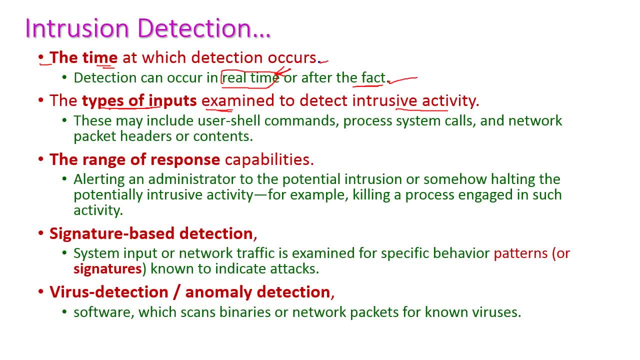 input should be examined to deduct intuitive intrusive activity. that is, the inputs includes the user shell command process, that is, system process call and network packet headers or the contents of network packet. so these may be the types of input to examine the detection system and the range of response capabilities here altering, that is, alerting. 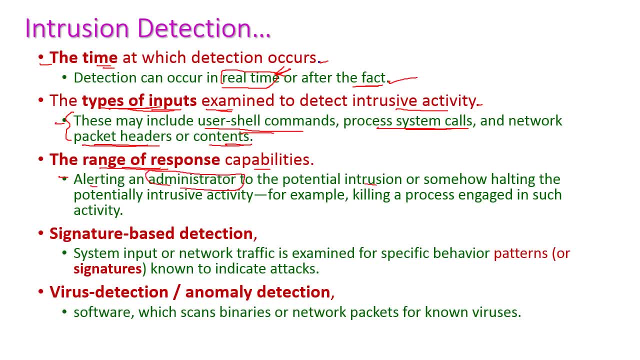 the administrator to the intrusion, um, or sometimes halting the intrusive activity. okay, by which process the intrusion taken place? so identify that particular process and killing that process so that the administrator will be alerted or safeguarded. and next one is signature based deduction. here the input or network traffic is 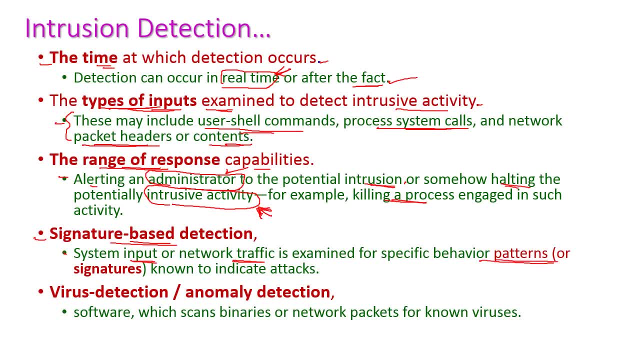 examined for a specific pattern or the signature known to indicate attack. okay, so this is very powerful. uh, intrusion deduction system. okay, signature based deduction. so they are going to monitor the behavior pattern or the signature of inclusive activity? right, and so are looking at universities titled הה. 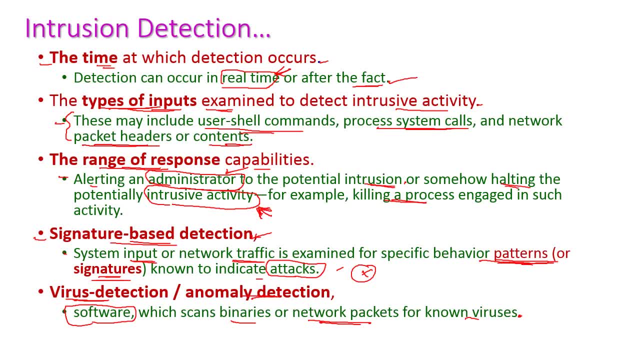 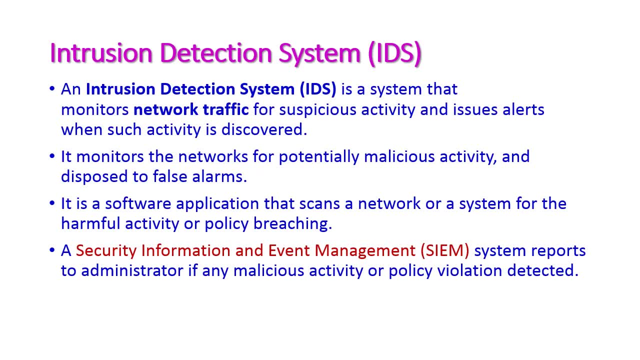 is mighty similar to the computer system. okay, to the system menu here. this to theика discussion today in person on dei voie. It monitors the computer system or network traffic for suspicious activity and issues alert when such activity is discovered. That is, this IDS will give the notification to the administrator if there is any malicious attack is happened in our system. 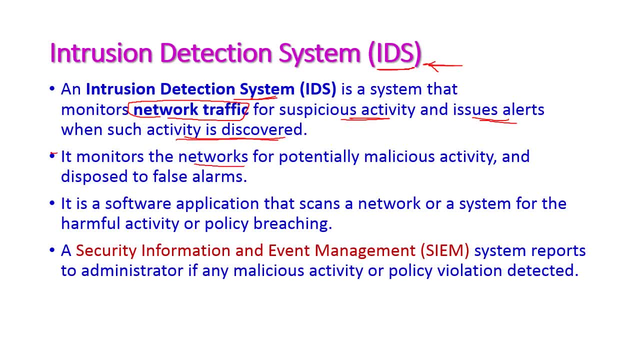 And it monitors the network for potentially malicious activity and dispose false alarms. And this IDS is a software application which scans the network or a computer system for the harmful activity or any policy breaking. If there is any harmful activity or breaking of policy, then immediately this IDS will alert our system administrator. 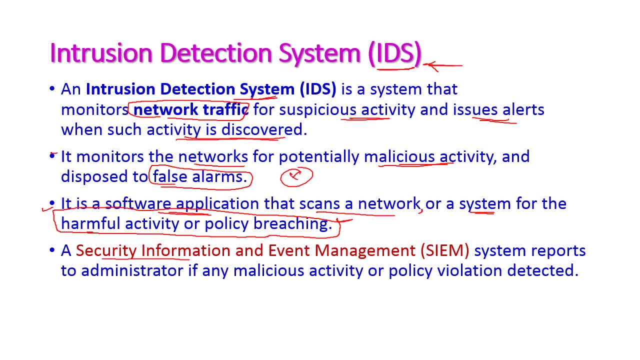 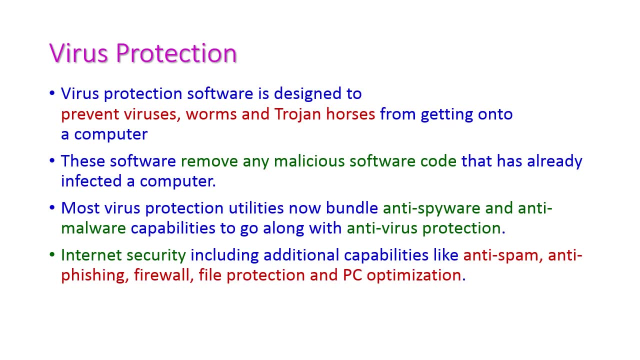 And it uses the security, information and event management that is, SIEM system, which reports the administrator if any malicious activity or policy violation detected. The next one is virus protection. This is a software, which is otherwise called as antivirus software, designed to prevent viruses, worms, Trojan horse from getting into our computer. 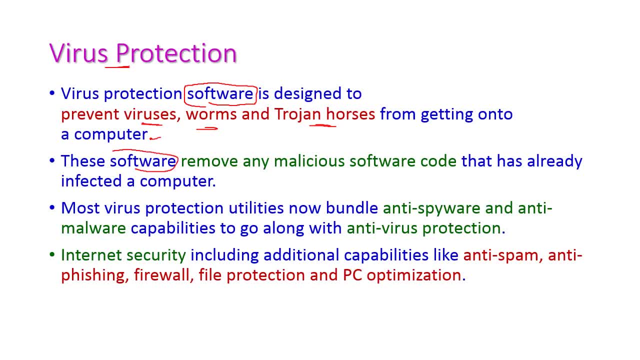 Right, And these softwares also remove the malicious code, that is, virus code, which are already infected our computer system And the most virus protection utilities bundled into anti-spyware and anti-malware capabilities and, along with this, antivirus protection. Ok, When come to internet security. 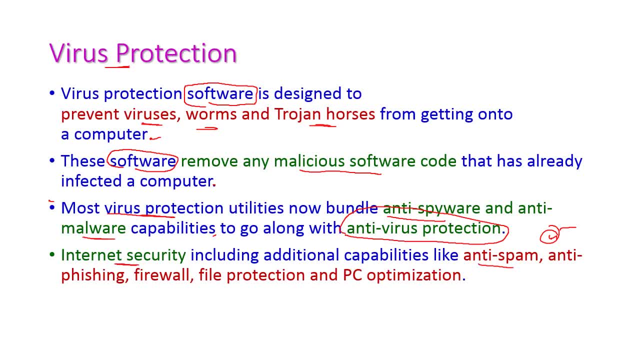 it includes some additional capabilities like anti-spam, anti-phishing, firewall and file printer, internet security And after some time it is ready to do the work protection and PC optimization. So these things will be included into this internet security. 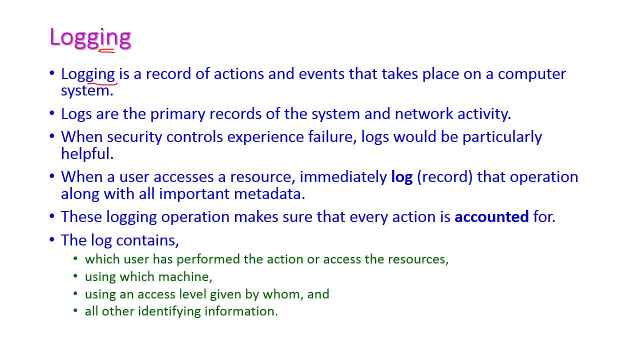 The next one is logging. Logging is nothing but recording all the actions and events which are taken place in the computer system. okay, that is called as logging, which is otherwise called as a record. okay, which records all the transactions in the computer, And logs are primary records. 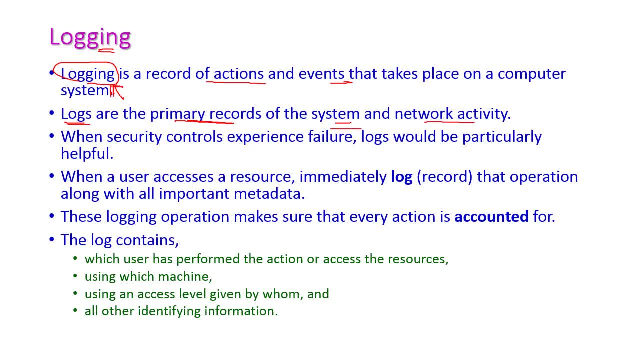 of the system and network activity. okay, this is important, right. When security control experience failure, then the logs would be particularly helpful. Then we can easily refer from the previous record and we can try to rectify our failures. And when user access a resource. 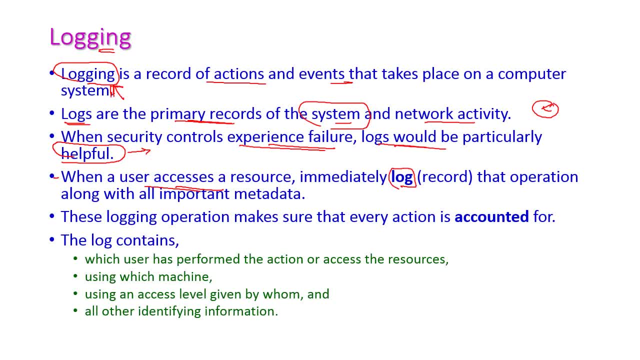 immediately. that will recorded into the log, and all important metadata should also be recorded into the log. So this is important, So this is important, So this is be recorded into that log. okay, these logging operations make sure that every actions is accounted for. okay, the the log record contains which user has. 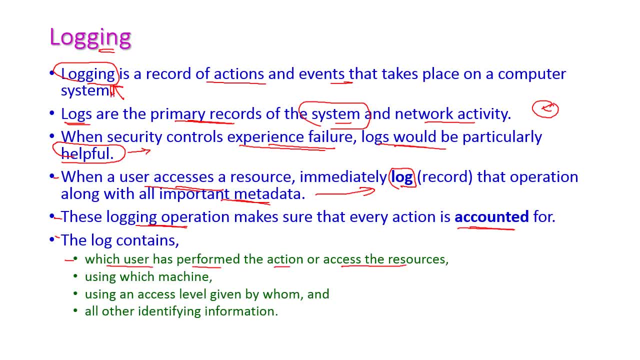 performed the action or access the resources and using which machine: the the user is accessing a resource and using an access level given by whom, and all other identifying information. so everything will be recorded into the log register. the next one is accounting. this is another potential tool in 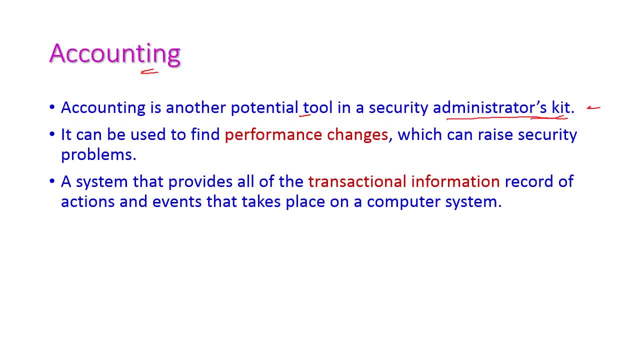 security administrators getting and it can be used to to find the performance changes which can do any kind of work and can be used to do that. so this is also called log register, can be used to to find the performance changes which can do any kind of work and. 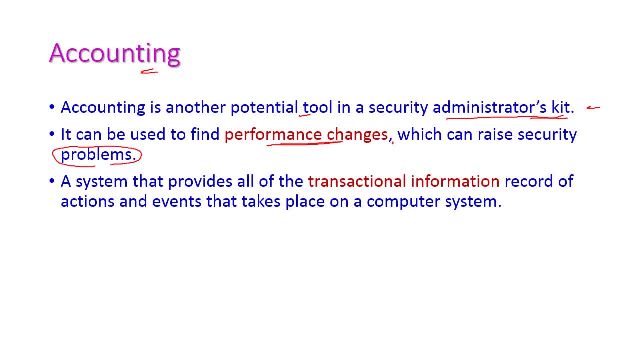 do any kind of work and can be used to to find the performance changes which can raise the security problems in our computer system. If there is any performance changes, then immediately we can find by using this accounting, and this accounting system will provide all the transactional information which are the records of actions, events and that will be taken place. 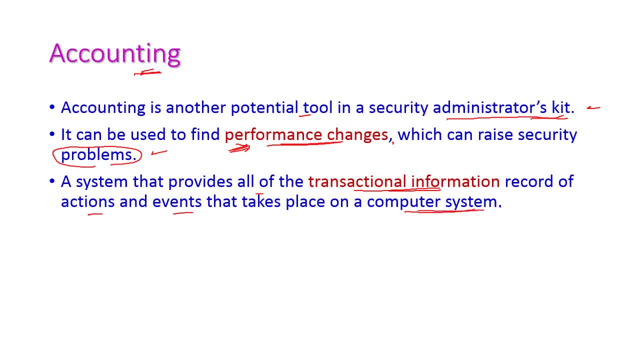 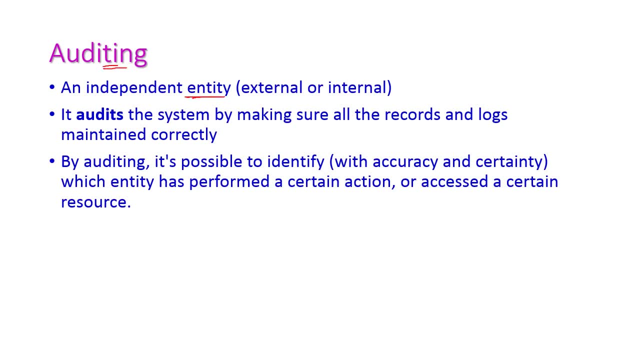 in the computer system or the network system. The next one is auditing. Auditing is independent entity or autonomous entity. There are two types: internal to our system or it may be external to the system and the auditing that will audit the system by making sure all the records and logs. 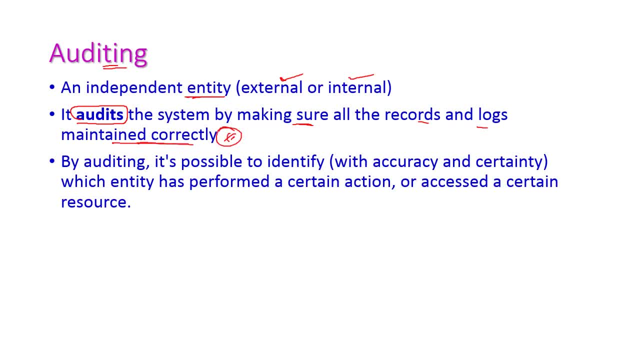 maintained correctly and by auditing we can easily identify with, accurately and certainly, which particular entity has performed a certain action, or which particular entity accessed, and which particular entity has performed a certain action, Certain resources of the computer system or the network system. okay, for this purpose we can use